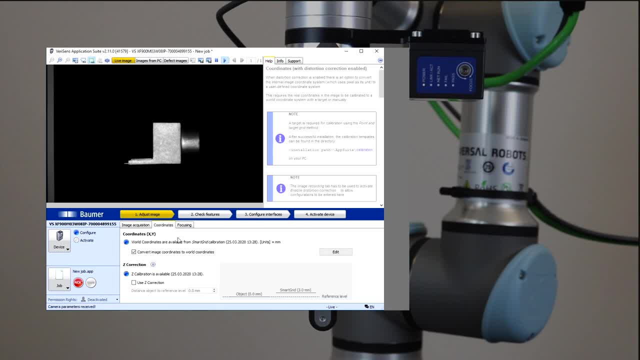 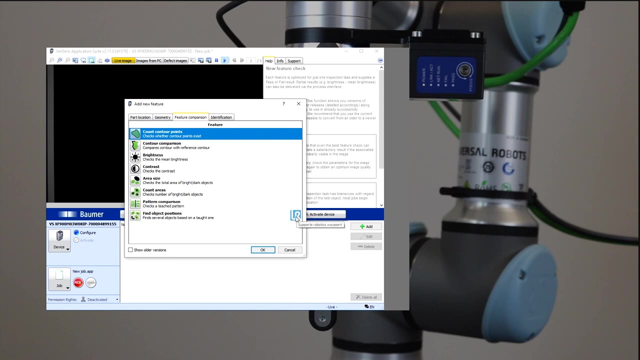 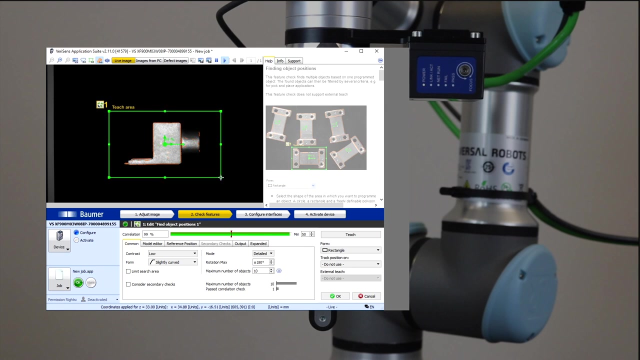 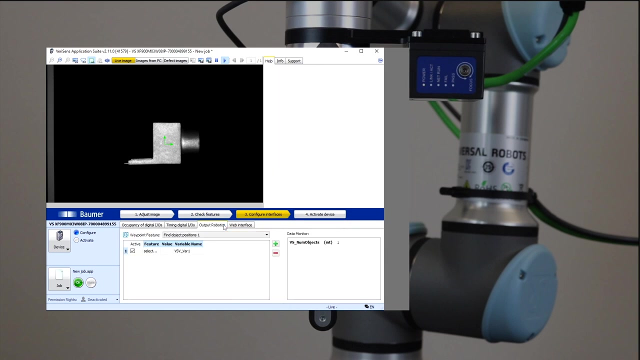 Next select the appropriate feature. check In the example. it's find object positions for contour-based identification of several objects in parallel. A small logo indicates coordinate transmission directly to the robot. These coordinates being the only data transferred eliminates the need for interference configuration. 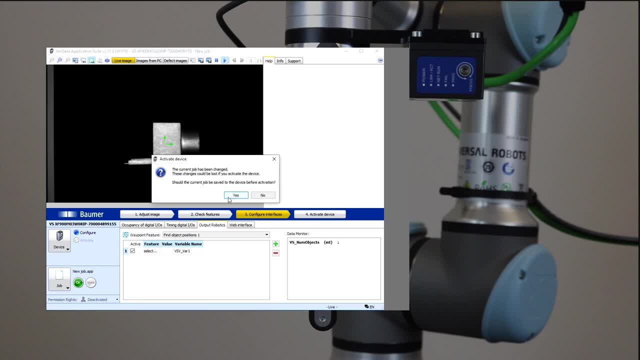 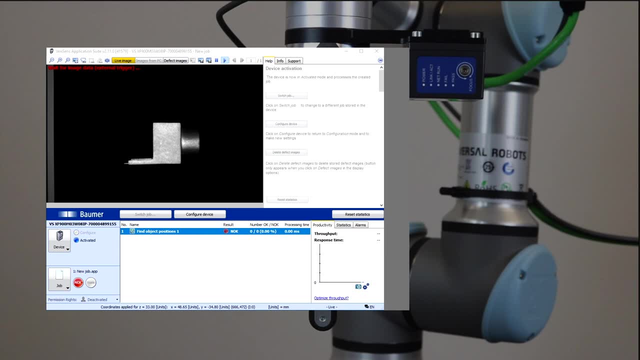 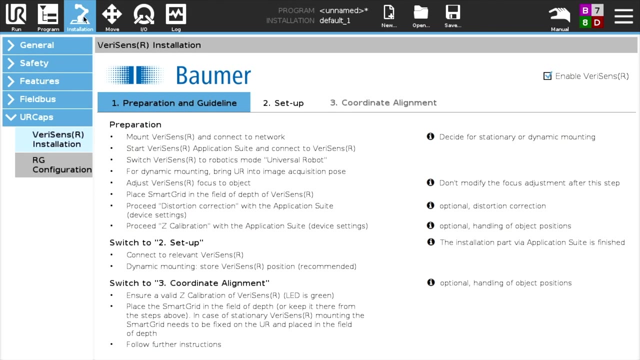 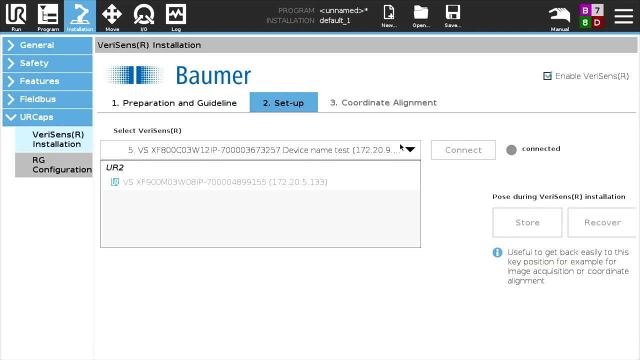 In the final step, VeriSense is activated, along with saving the job. VeriSense UR cap has already been installed via USB stick in the robot controller. Step one explains how. Second step is selecting and connecting the configured vision sensor and also saving the current robot position. 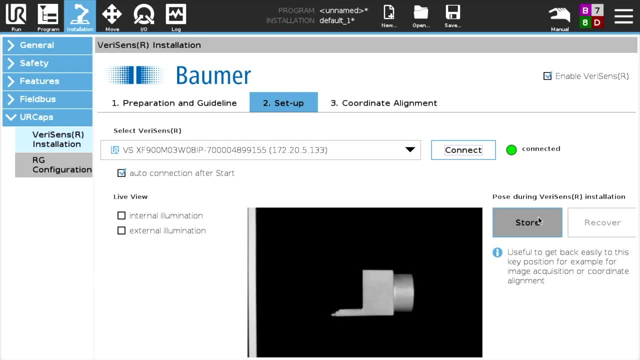 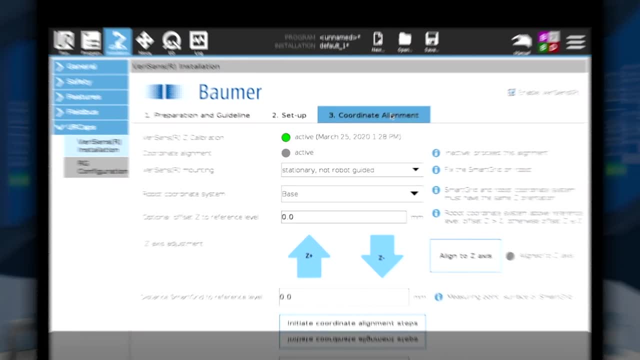 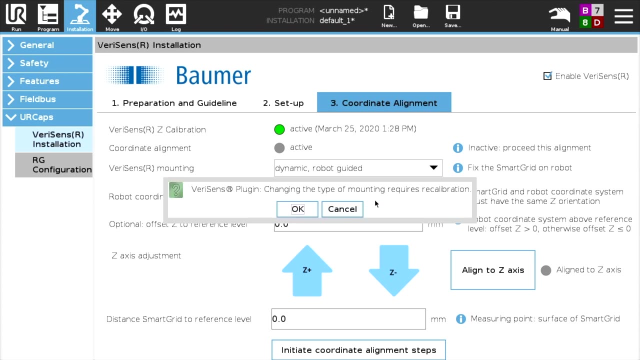 Step three is only required for image-based coordinate approach, as in the example. If all settings are correct, the LEDs light up. If all settings are correct, the LEDs light up. More settings are application specific. The last button is for call-up the coordinate alignment. 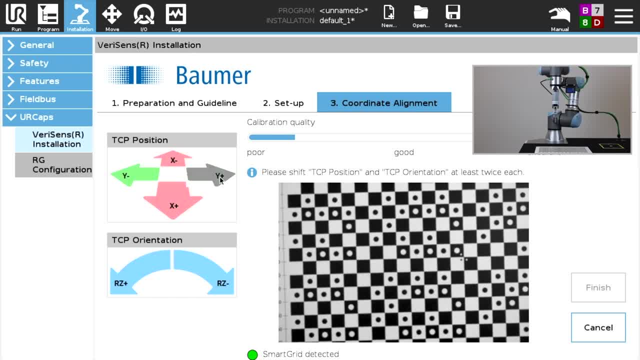 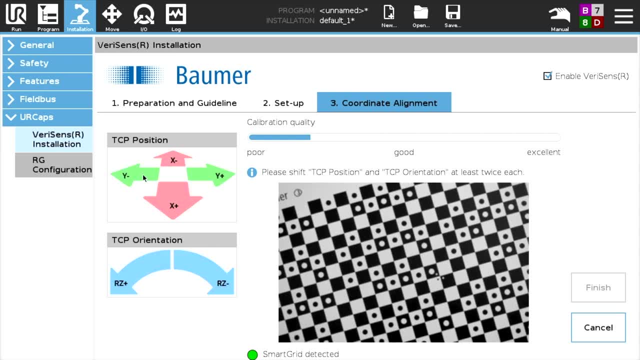 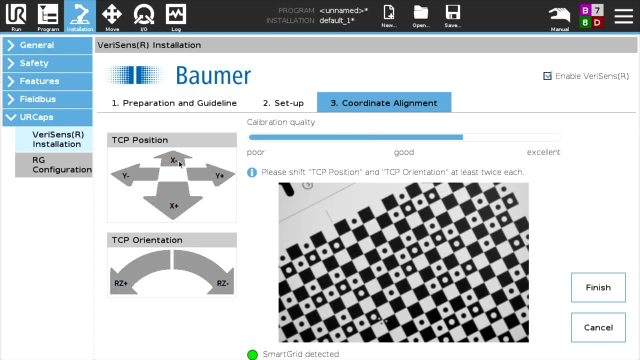 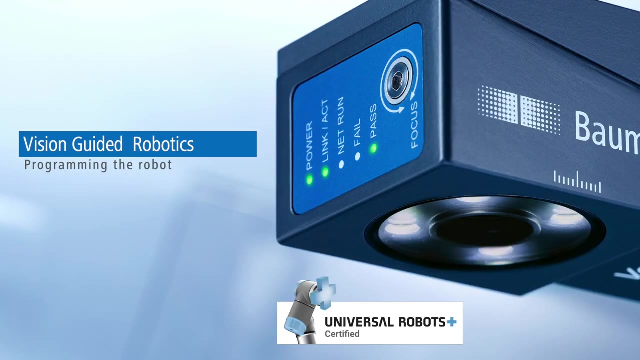 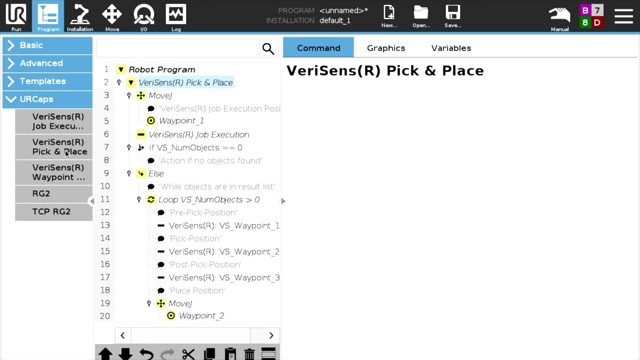 SmartGrid requires only few linear and rotational movements to ensure a good calibration quality, without the usual hassle of multiple, error-prone and manual calibration. 가요 Now it comes to robot programming to ensure reliable submission and placement of objects. In order to ensure reliable pick-and-place of objects, 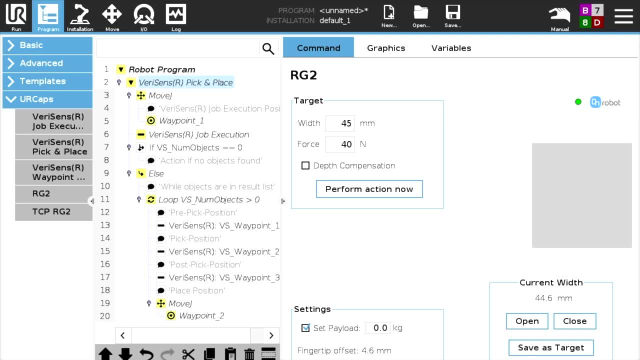 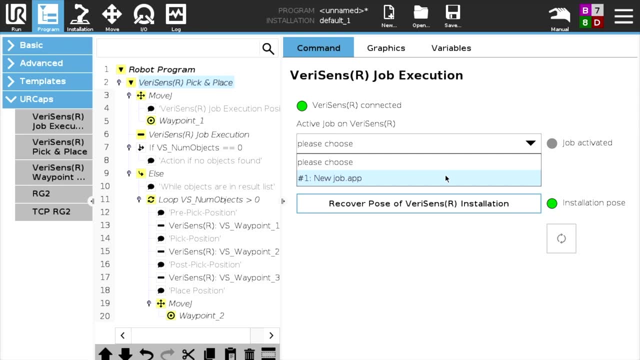 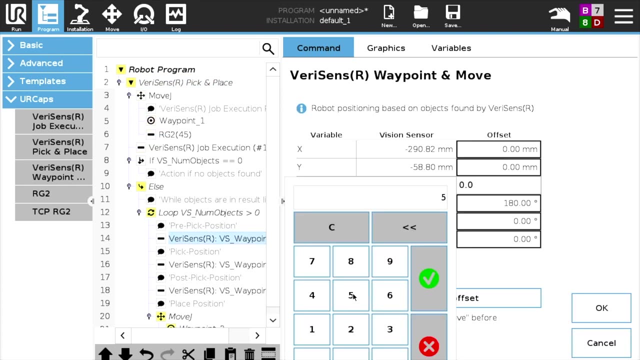 In order to ensure reliable pick-and-place of objects. in order to ensure reliable pick-and-place of objects- I am sorry, VeriSense job execution is for image acquisition and retrieving results. VeriSense waypoint and move is for coordinate approach via image-based waypoint.